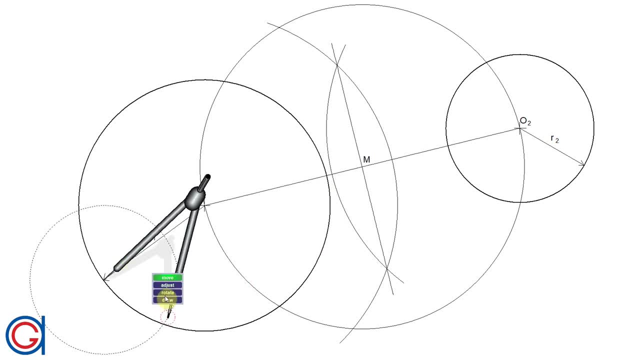 our compass on the length R2,. we are going to transport it onto the extremity of radius R1, as can be seen here, And the distance left between the new point to the center point O1 is the difference between radius R1 and radius R2.. So now setting our compass on radius 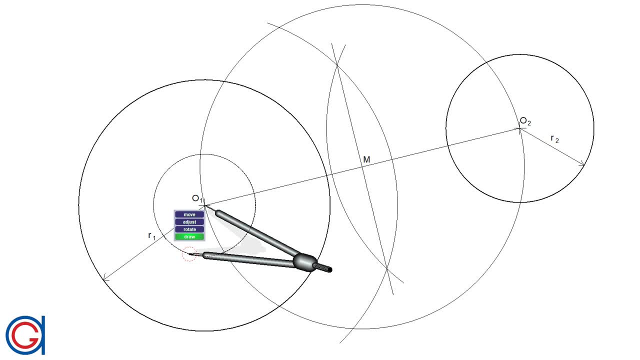 R1 and with length radius R1 minus R2.. We're going to draw another circle And, as you can see with the red dots, it cuts our previously drawn large circle at two points. So the next thing we're going to do is with: 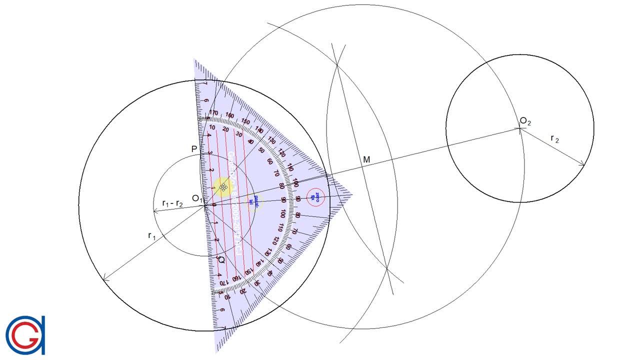 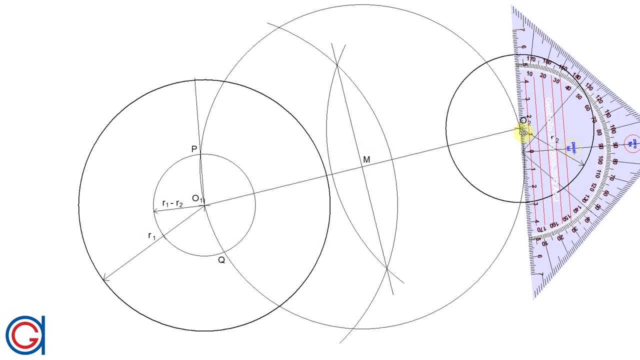 a ruler. we're going to draw a line from O1 going through point P and elongated until it touches the given circle at our first tangent point, T1.. And now we're going to draw another line parallel to this point, O2, until it touches the outside of the circle, which will be our second tangent point. 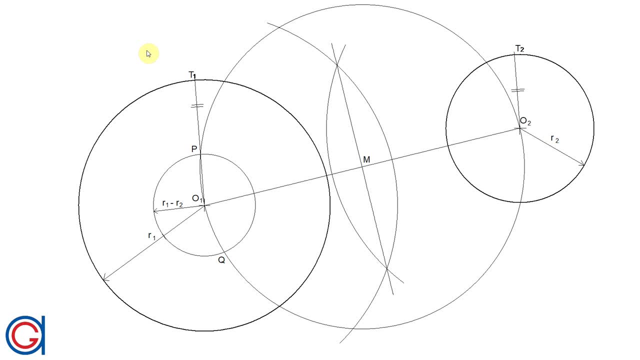 T2. and now we're going to repeat the process on the bottom sides of the circle, joining O1 through point Q until it touches the outer circle at our third tangent, point T3. and again we will draw another parallel line to this from O2 until it touches the outer circle at our fourth tangent. 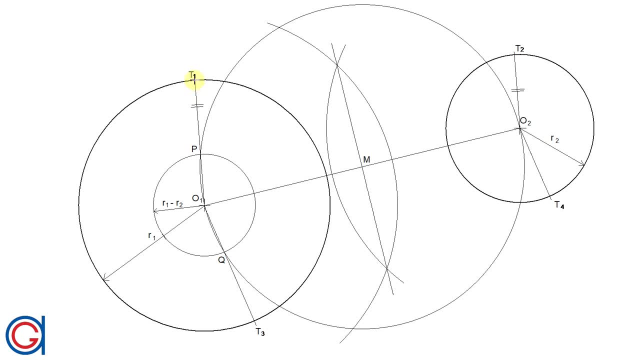 point T4. so now, with a thicker line, we will join tangent point T1 to T2, as can be seen here, and tangent point T3 to T4. and now, just to complete the drawing, we're going to use a thicker line setting the compass to the radius O1 R1. we draw with a thicker line to complete the drawing. 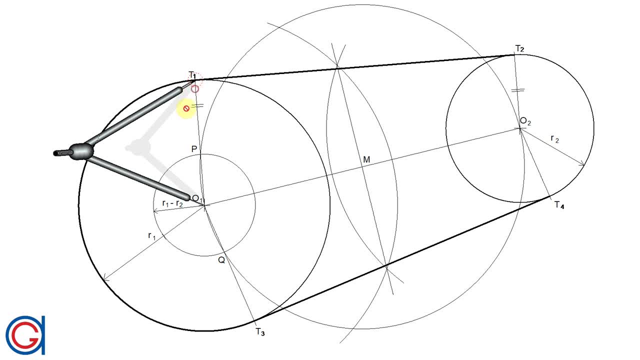 and the same setting the compass to radius R2 with a thicker line. so you have a spectral governor and now we're going to join tangent point T2 to T1. so by doing this we'll circuit, or a chain of a bike, and now, with a 45 degree set square, you can see our 90 degrees. you. 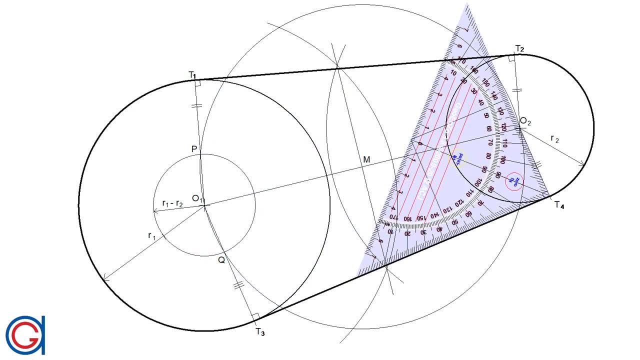 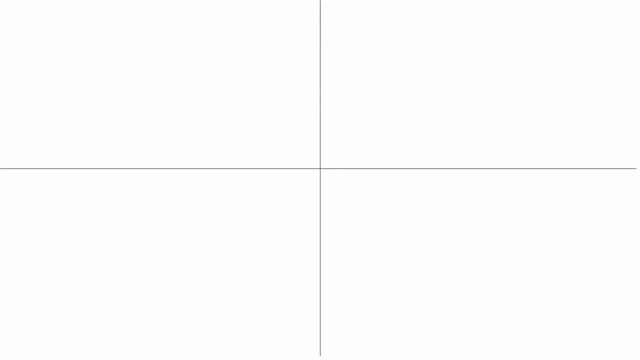 can see, checking that all our angles are 90 degrees and we mark our parallel lines also. so i hope this video has helped you. please press like and subscribe to our youtube channel. thank you, until the next video, you.